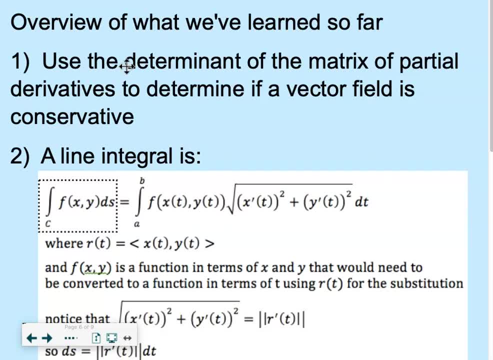 But we also learned how to use the determinant of the matrix of partial derivatives to determine if a vector field is conservative. That was the test for whether a vector field is conservative or not. If a vector field is conservative, it means there's a potential function, and we all know how to do it. 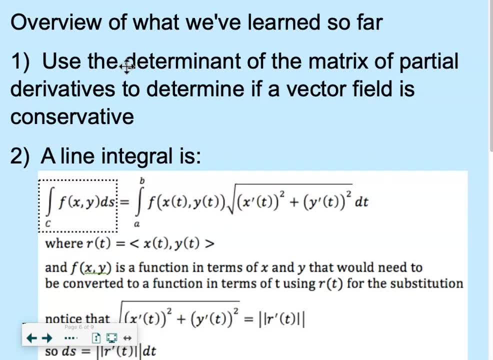 But we're working on how to find a potential function. All right. First definition of a line integral that we learned was in terms of arc length, right, So it's just an integral over a curve C of some function with respect to arc length. 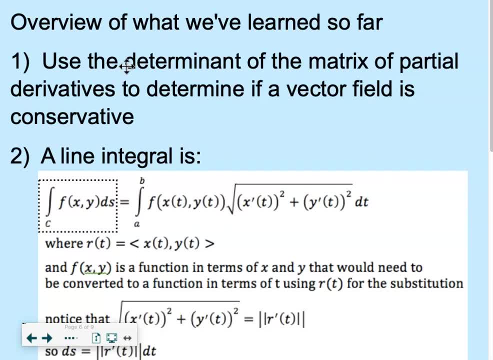 So when you actually convert this To a DT integral, you have: Ds becomes the square root of X prime squared plus Y prime squared DT, And your F just gets written in terms of X of T and Y of T. So you're replacing your Xs and Ys with functions and sums of Ts. 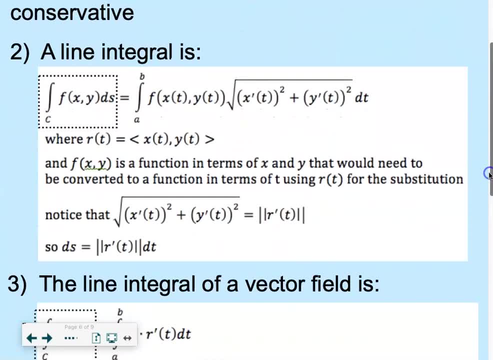 So first line integral that we learned was, with respect to arc length, Couple of things to notice. I don't know if you remember this or not. Arc length is the magnitude Right, It's magnitude of the speed, the magnitude of the velocity. 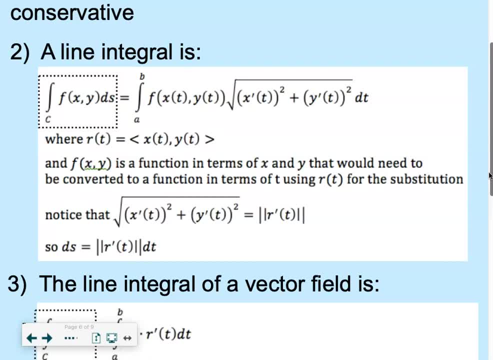 This right here. this is our definition of arc length: the square root of X prime squared plus Y prime squared. That's for a little inspiration, But anyway. So it's the same thing as the magnitude of R prime, And so Ds is equal to the magnitude of R prime. 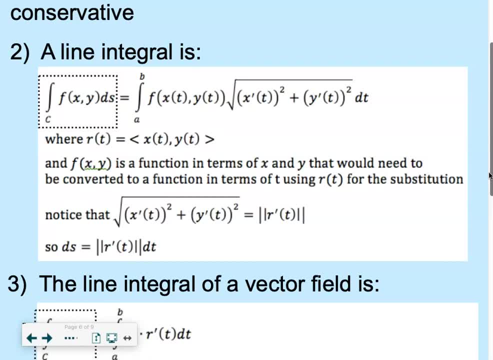 You just need to remember this. There's nothing wrong with this, It's just F, Alright. Well, thanks, Bye, Bye, Bye of our prime DT and it's kind of a conversion formula. you can almost think of the magnitude of our prime slight digit. oh yeah, for converting those units. 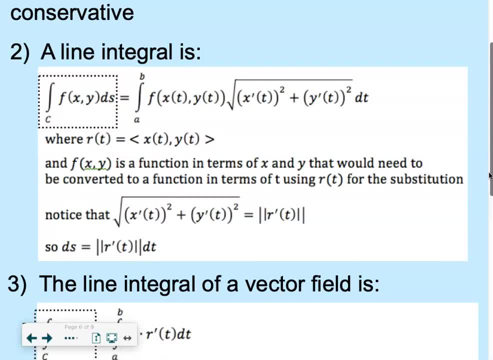 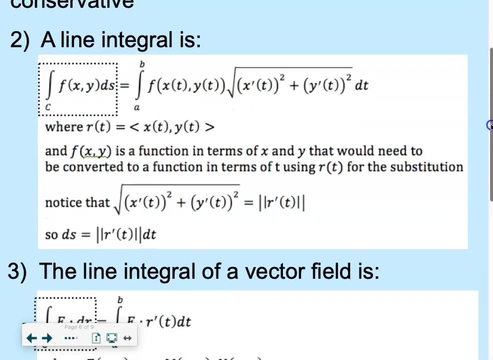 from SS 15. so anyway, so deep. it used to confuse me how we went from DS to DT, but it's because your DS is equal to the magnitude of our prime time. all right, line integral of a vector field. so that's traditional line integrals first. 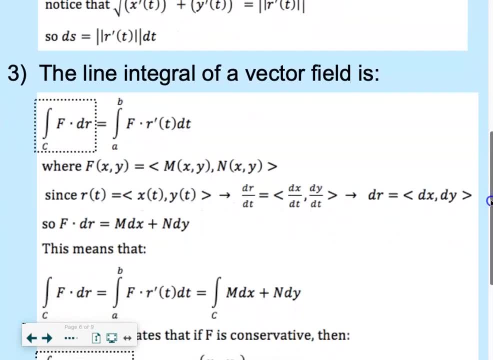 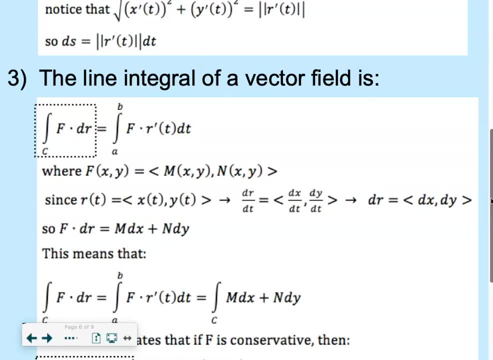 definition you like line integral of a vector field: F dot dr, which is the same as F dot, our prime DT. so so dr is the same as our prime DT. all right, so F. if we write F as M comma n and R as X comma Y, then F dot dr equals MDX plus N dy. why? 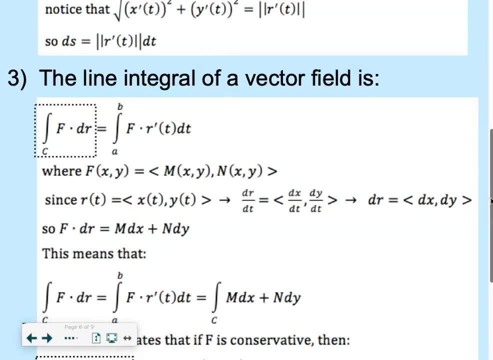 at this point we're going to be able to write F as M comma N and R as X comma Y. this is where I was talking to you guys yesterday and I think I would show you a little bit of a conversion. so, dr DT, right, that's our. dr DT is DXG TV. why T? 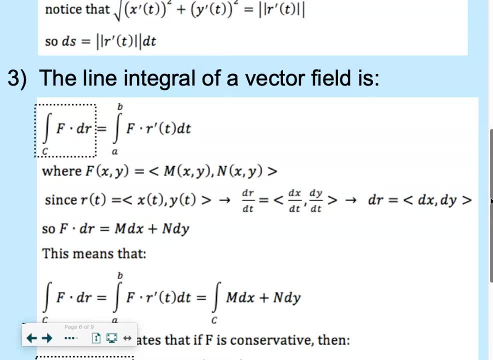 if you remove the DTS from the situation, you get dr equals DX dy. so if you do F dot dr, you get MDX plus M dy. so F dot dr is actually equal to. and yes, and why I'm- You can do the dt's, but the dt's all end up just canceling out. 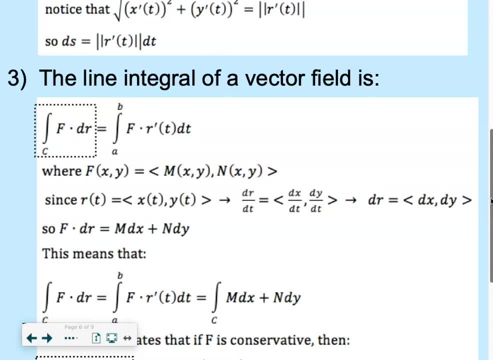 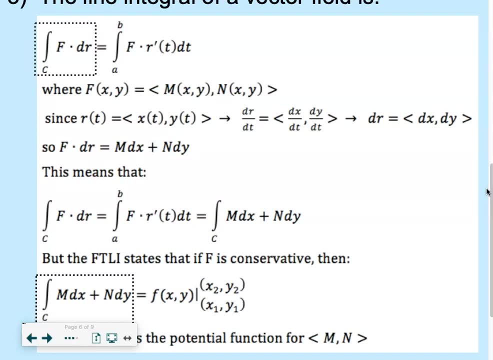 So it works out nicely. So anyway. so f dot dr is the same thing as f dot r, prime dt, which is the same thing as the integral of m dx plus n dy. So we did one that was like this, just with x's and y's normal. 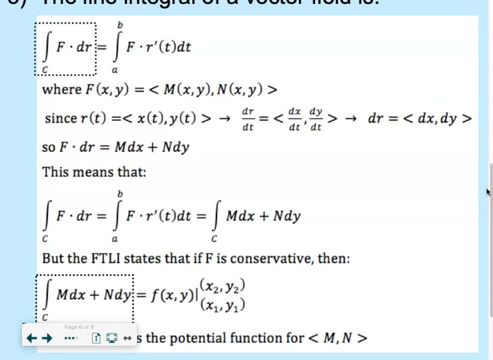 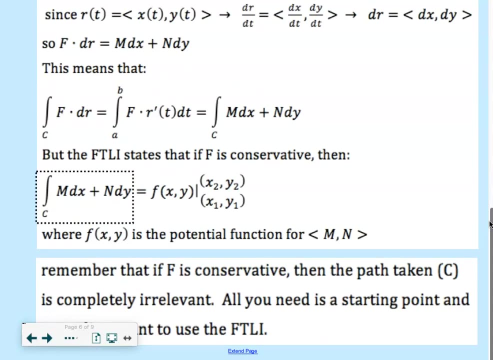 Then we learned the fundamental theorem of line integrals, which says that, hey, if your vector field is conservative, then the path to get from a to b is completely irrelevant. So why not just do the simplest path possible, which means find the potential function for big F? 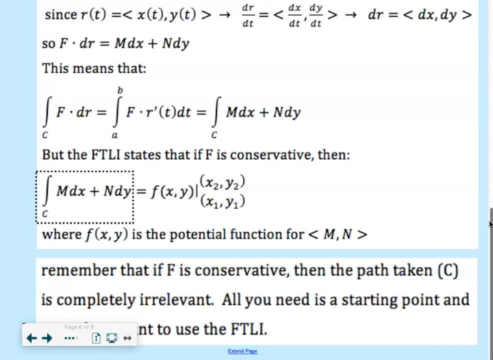 and then evaluate the potential function from beginning point to ending point And you end up with an equivalent value for your f dot dr. All right, So F-T-L-I fundamental theorem of line integrals says that if F is conservative, then the integral over curve C of m, dx plus n, dy. 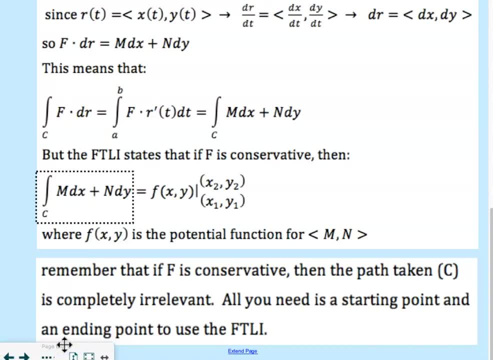 is equal to the potential function F. from point one to point two. Remember that if F is conservative, the path taken is completely irrelevant. All you need is a starting point and ending point to use the F-T-L-I. Okay, There's a little more before we get into problems again. 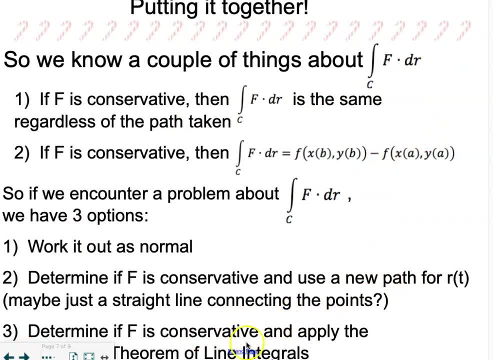 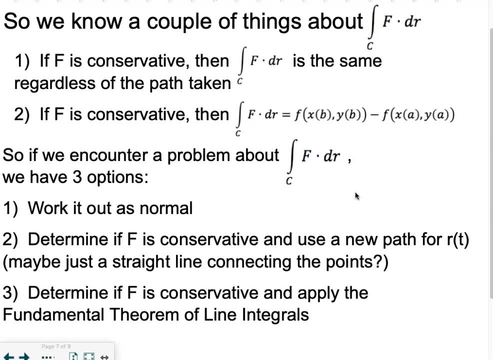 So I don't know if I can make this a little, I'm going to move this up, Okay, So here's the thing: If we have an F, dot, dr integral, then we know that if the vector field is conservative, then this integral is the same, regardless of the path taken. 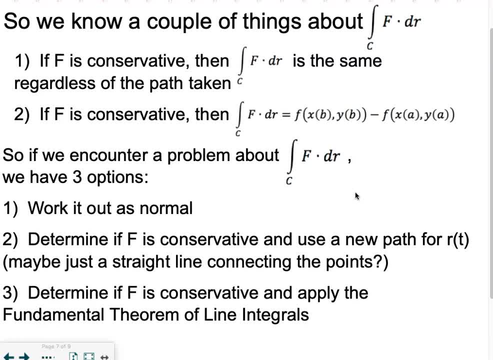 We also know: if the vector field is conservative, then this integral also equals the, the potential function from A to B. basically, So if we encounter an F dot dr problem, you have three options. You can actually find F dot dr Like you can do it. 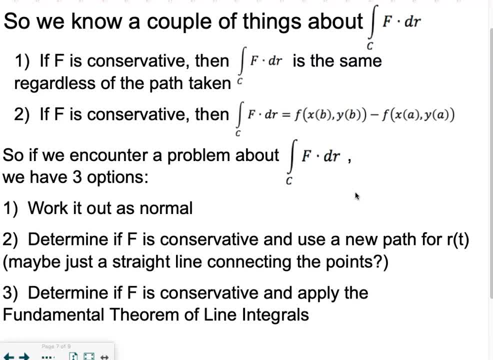 So you do the dot product of F and R prime and you know with respect to T's and you'll be good, Or you can find a new path right. You, your R of T say your R of T is some crazy convoluted path from point A to point B. 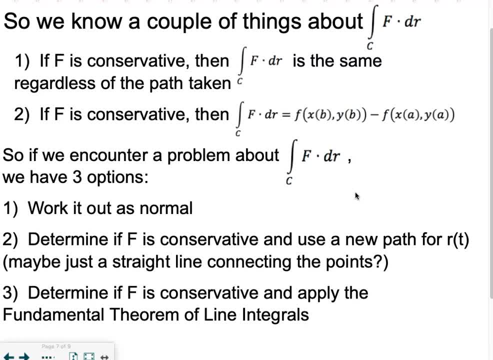 Okay, You could just make it a straight line from point A to point B and you'll get the same value for the integral, Or you can use the fundamental term of line. So you have options for your F dr problems, All right, And then today you're going to learn options if your vector field is not conservative. 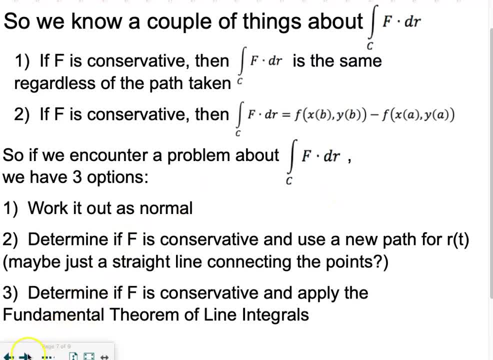 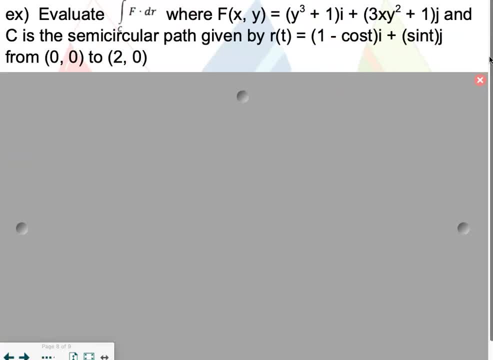 So we've now. we've got options, easy options if the vector field is conservative, And then after today we'll learn options if the vector field is not conservative. But before we do that, let's just practice Real quick. So I want you to find F dot, the line integral of F dot dr, where the vector field is Y cube plus one for in the X, for the X component, and three X Y squared plus one for the Y component. 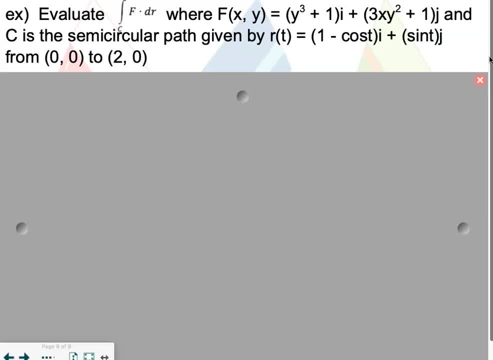 C is the semi circular path given by that R of T, one minus cosine T in the X component and sine T for the Y component, from zero zero to two zero. So the first thing I personally would check would be to see if F is conservative, because if F is conservative, 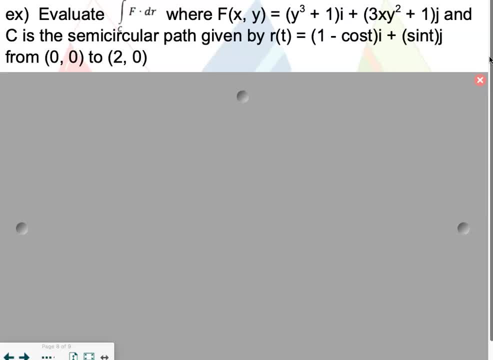 then you can do this using either changing your path or doing F, D, L, I. if F is not conservative, then you got to do the old fashioned. So take a minute I'm walking through, just for the sake. I'm going to walk you through the three possible ways you can do this problem. 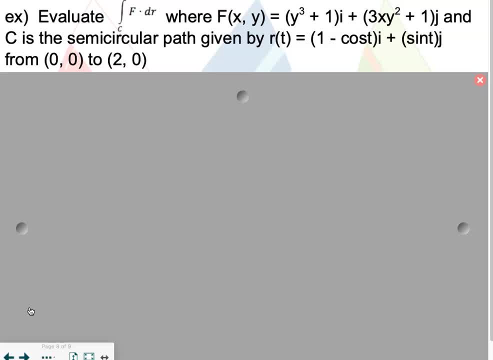 So way number one is to go ahead and do F dot R prime. right? If you go ahead and just do F dot R prime, then you have to rewrite your F where it like this: if this is your X and this is your Y, 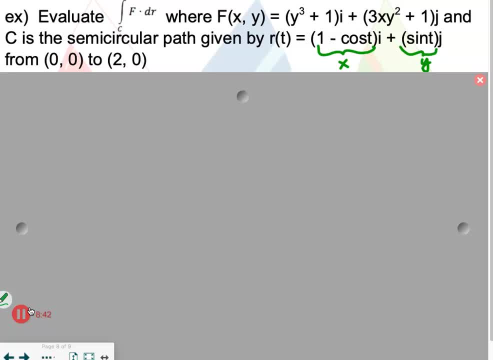 right, You'd have to replace this, So this would be sine Q plus one, and this would be three times, this times the squared plus one, and then you would do the dot product of this vector and this vector, right, And then it's great that you could do that. 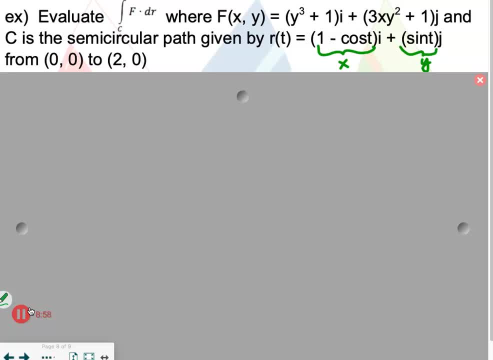 It is a lot of work. Yes, So that's method number one. Method number two: Did anyone test to see if BDF was conservative? Is it conservative? Yes, Since BDF is conservative, you can. you have two options. 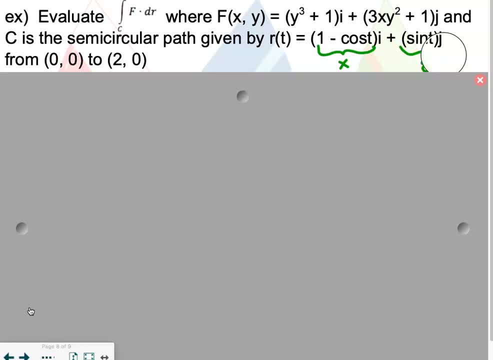 One is you can change your path right. So currently we're following this R of T to get from zero zero to two zero. but we could just as easily follow R of T equals T comma zero from from zero to two and do the exact same problem. F dot, R, prime. 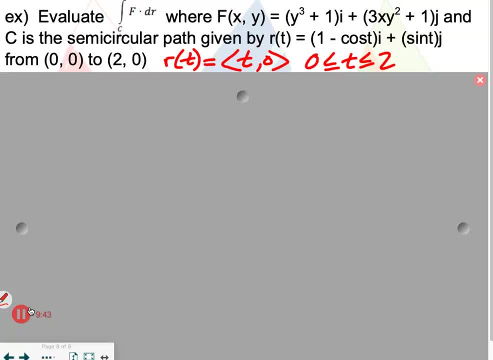 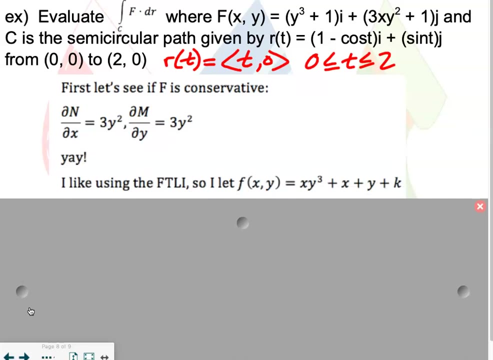 which would be much, much easier, right? So you could do that, or you could use the fundamental theorem of line integrals. I personally like the fundamental theorem of line integrals the best. So first you have to find your potential Function, right. 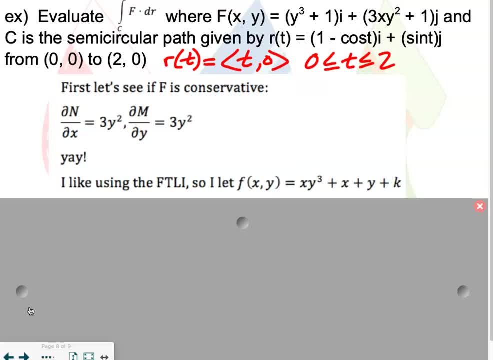 So do you guys need me to walk you? I'm happy to walk you through. Do you want me to walk with your finding essential? Yes, Okay, All right. So potential function for F. So our little app. So you integrate Y, Q plus one with respect to X. 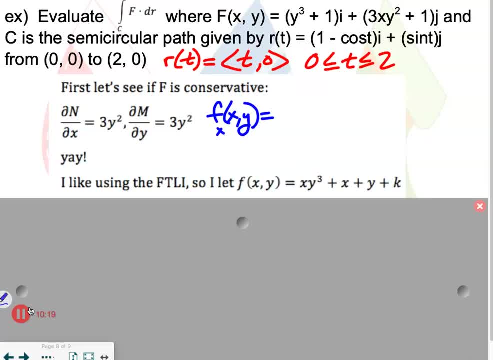 So I'm going to put, like this, little X here, So we have X, Y, Q plus X, and then you do the same thing with your One- I'm not writing. So you do the same thing with your Y part. You integrate the second part with respect to Y and you get X, Y, Q plus Y. 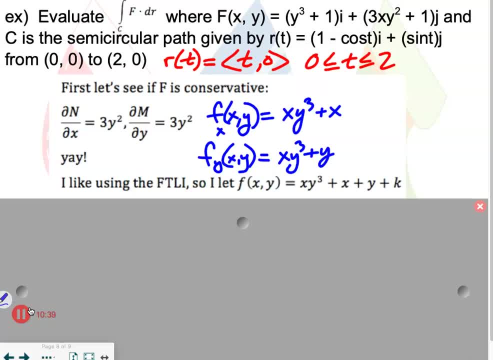 And then when you write your potential, it's all of these terms, but without We have an X, Y, Q plus an X plus a Y. Okay, So there's your potential function and then all that. the fundamental theorem of line integral says: 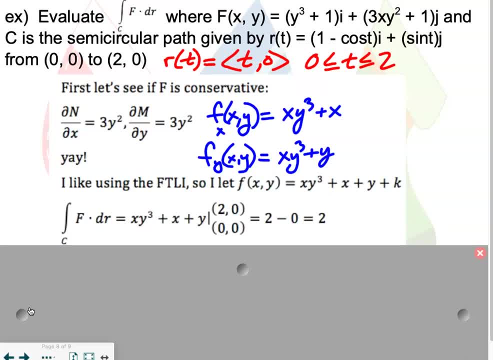 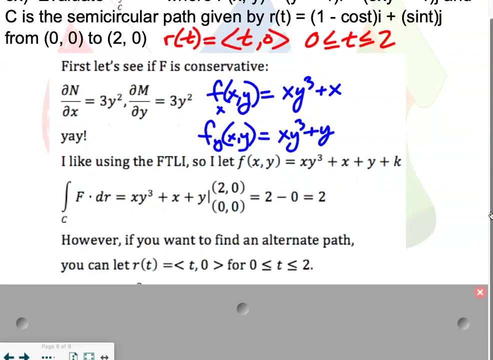 is that the integral of F dot DR is equal to the potential function evaluated from beginning point to end point. So you plug your end point in minus. plug your beginning point in and get your answer and you're done, Right? Yeah, So this was me doing it using the R T T comma zero. 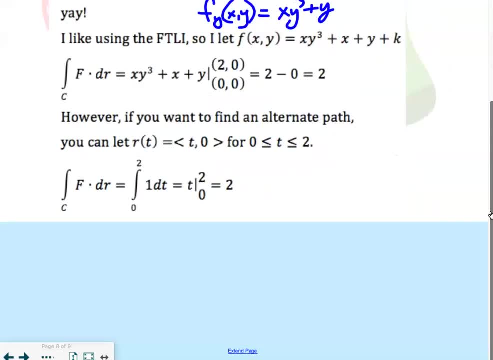 And I actually Worked it out both ways so you could see that it actually works both ways. It's really like when you change your R T. look at how easy being able to come right. So this way is really no harder than F T L I. it makes it really nice. 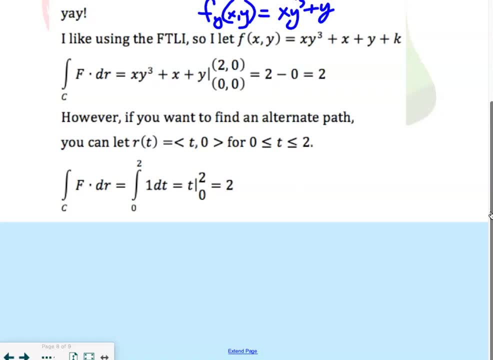 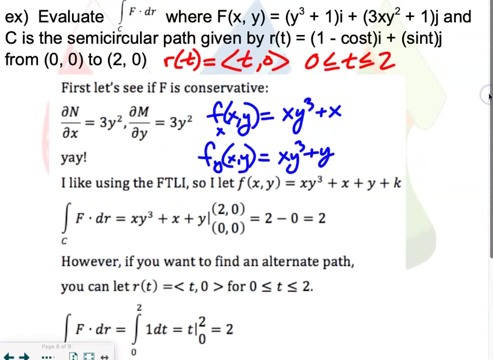 So as long as the vector field is conservative, you can get from point A to point B on any path you want. as long as it's a path that works, We'll have an equivalent. All right, Any questions on that one? Just, you have a question. 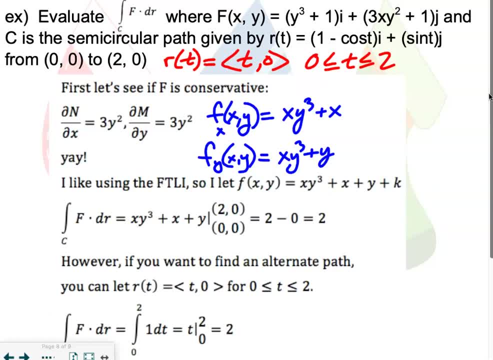 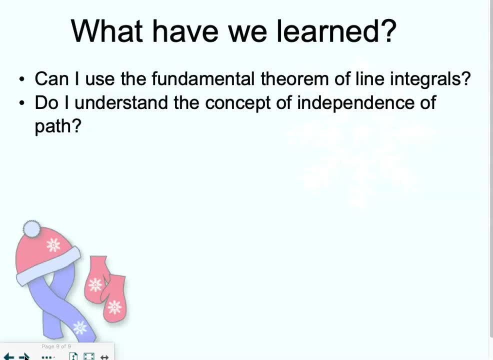 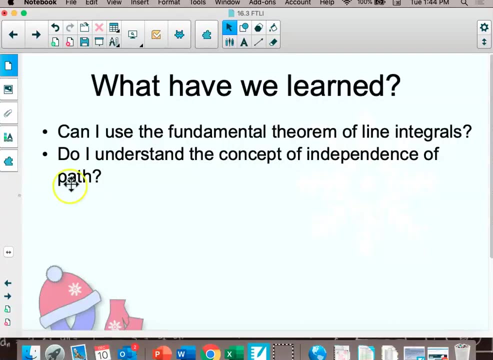 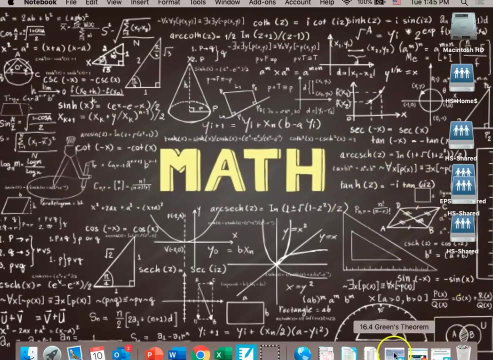 For sure, Yeah, All right, Okay, So that's it for this lesson. That was all we needed to do to finish off fundamental theorem of line integrals. Now we're going to switch To The Green's theorem, And I do have a warm up. 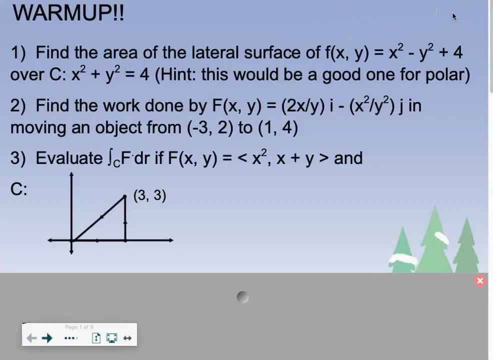 And I think I want us to take about five or ten minutes and do the warm up, because it's a good review. So Your first question: Find the area of the lateral surface. This is not a work problem, So you might. You are going to just have to do this using a traditional line integral. 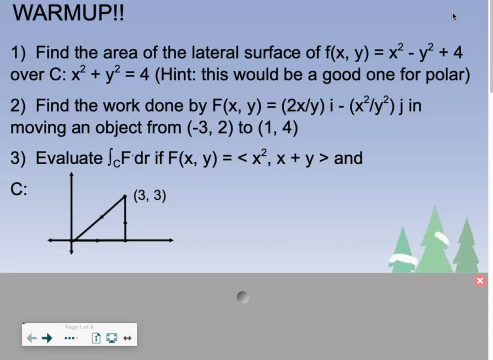 It's just going to. It's my way of forcing you to use To find an old fashioned one, Right? So Find the area of the lateral surface. If you're f of x, y is x squared minus y squared plus four over the curve, x squared plus y squared equals four. 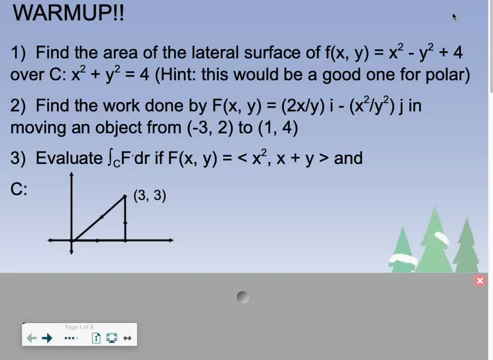 So you're just following along a circle with that as your height Right. Okay, Part two: Find the work done by big f of x, y- Make sure you check to see if it's conservative. And part three, Evaluate f dot dr. 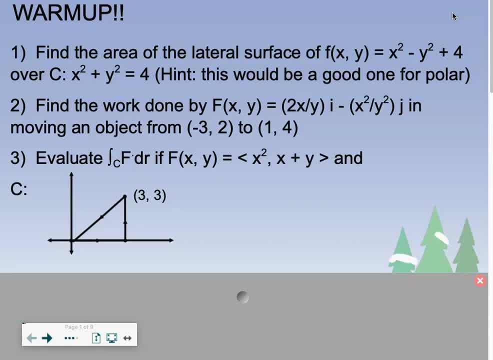 If f equals z. Again, I would check to see if it's conservative- It might be, It might not be- So if it's not, then this could be my way of forcing you to have to find parametric functions for these things. 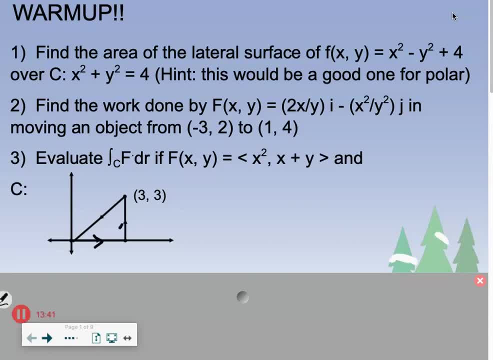 Yes, So the arrows look like that. that. that All right. All right. I mean a lot of good discussion on this problem. I enjoyed walking through this with quite a few of you. So Find the area of the lateral surface of f of x, y. is x squared minus y squared plus four over the function c. 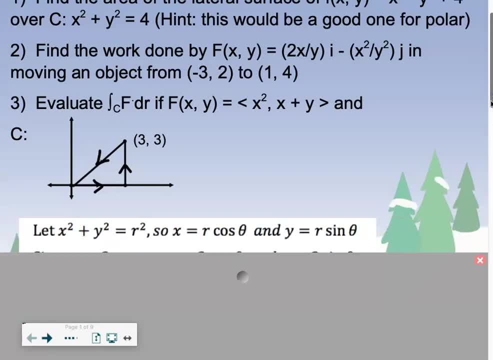 This would be a good one for a polar. So So I let x equal r cosine theta, r sine theta, And since our r is two, you get two cosine theta and two sine theta. So then you have to rewrite your f in terms of theta. 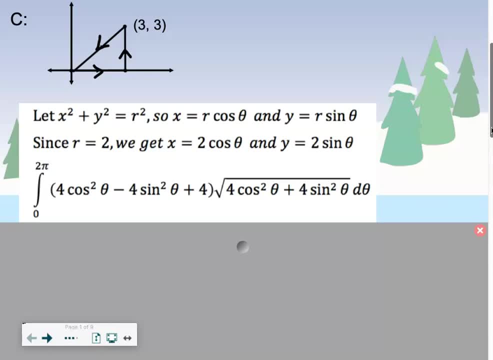 And you have to multiply it by the arc length of r Right, So you end up with square root R, root of four, cosine squared, plus four sine squared, which is root four, which is two, And you can pull out a four out of each of those and put an eight out front. 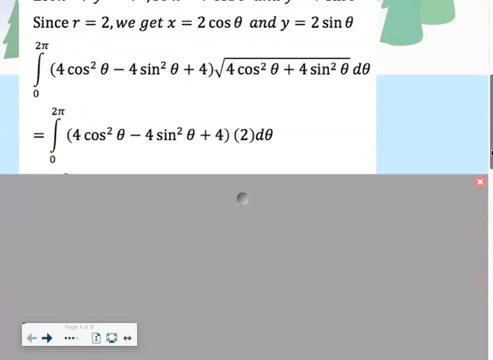 But anyway, so you end up with that. And then I pulled out an eight. Okay, This is where some people got stuck. I would rewrite cosine squared minus sine squared as cosine two theta. Some of you just did power reduction on both of them. 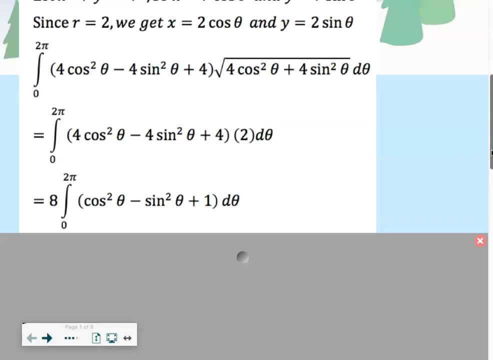 If you do power reduction on both of them And combine like terms, you still end up with cosine two theta. So no matter how you do it, you end up with a cosine two theta And then the anti-derivative of cosine two theta is one half sine two theta. 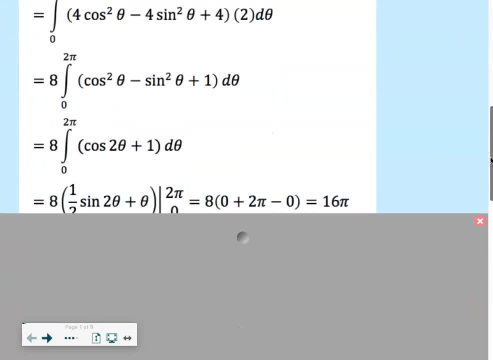 And the anti-derivative of one is theta. And then you plug in your two pi minus, plug in your zero and you end up with 16 pi. Somehow, I think you're coding this Coefficient Right at the beginning. I don't know. 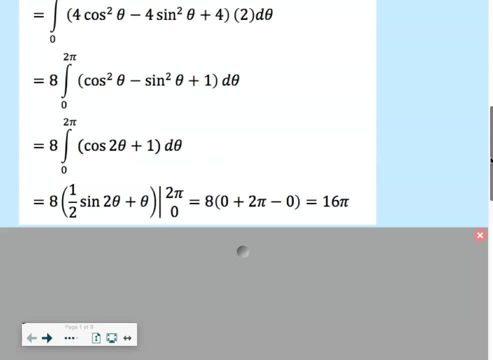 Four times two. You know what You have? four root, four on this step And the very next this right here. Oh no, that was the root of halves. You know what I found it? This is equal to one half times the life force of theta. 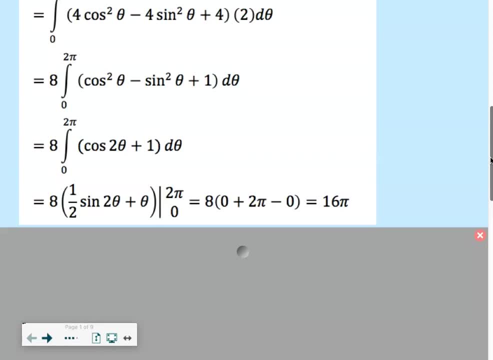 This is equal to one half times the life force of theta. One minus one plus one, Whatever. Okay, You guys. One divided by a half is not a half, It's two. So this should have been two, two, two, two. 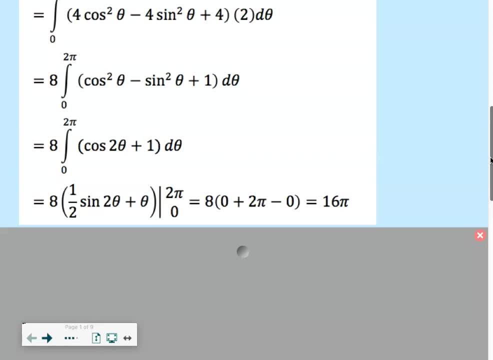 And that's where the problem is. Yeah, So a little mistake, All right. Good, Almost everybody figured that out eventually, which is really good. Are there any questions? Look at this. Look at all those beautiful 16 pi. All right. 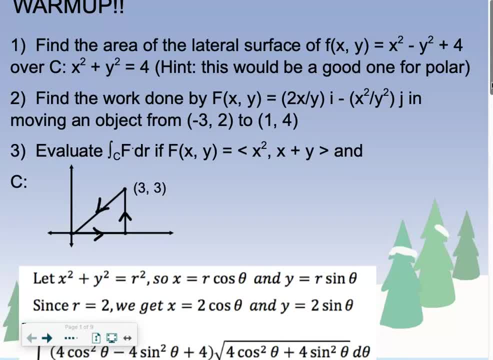 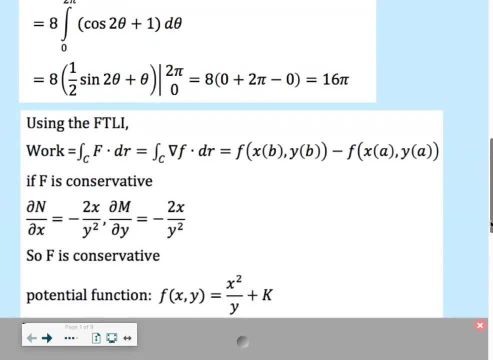 The next one, If you check It is: It is conservative, So I would have probably just done this with FTLI. And yes, yes, yes, It's a lot of work. I'm just Okay, And I got negative 17 fourths. 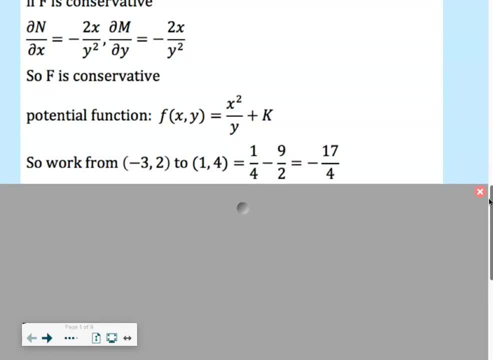 Negative 17 fourths. I see a negative 17 fourths. I see a negative 17 fourths. I see a negative 17 fourths, Like there's big banners around it And yes, we all got number two, So we all love fun. 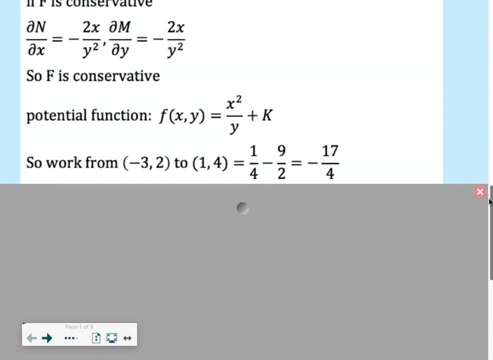 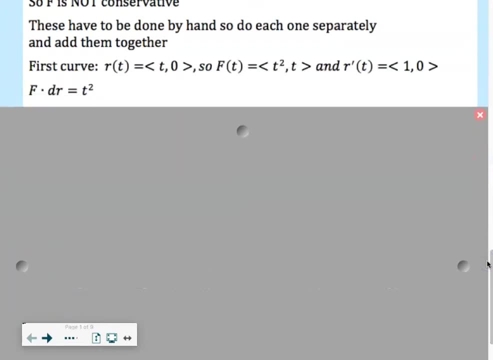 It's not an all-in-one right. Who doesn't love FTLI? All right, The last one. you had to rewrite your equations in parametric form, So I did each curve separately. So I did T zero for my first curve, probably from zero to three. 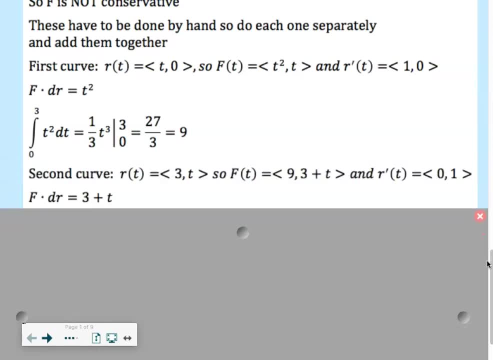 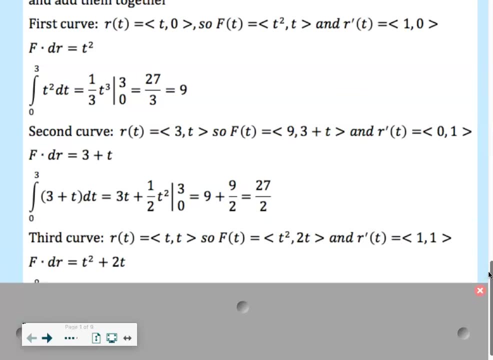 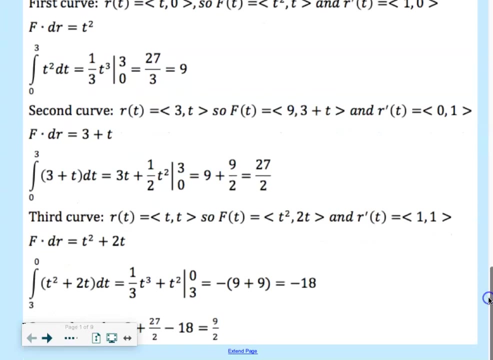 Yep, And then I did my second curve, which was three comma T, from zero to three again. And then I did my third curve, Which was T- T, And I did it from three to zero. I like was lame, So you could do that. 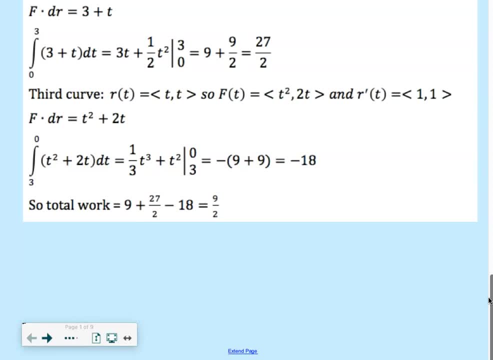 It's the same as doing negative T, It's the same thing as reversing it and making it negative, negative. two negative two. But anyway, or one minus T, one minus T, or three minus two, three minus two, Yeah. 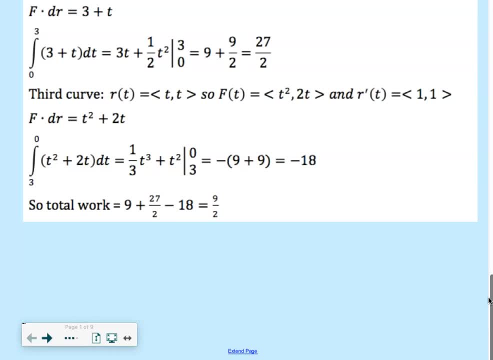 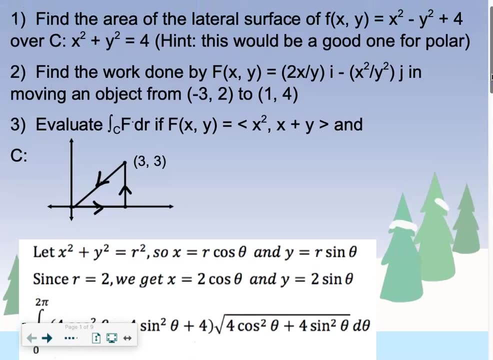 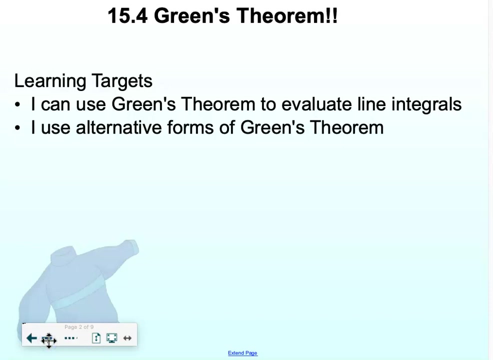 Both of them. Okay, Okay, All right. So that's enough of that. So we're going to move forward, And today we're learning green theorem Fifteen. Oh, I forgot to change again. I swear to you, I did go through these. 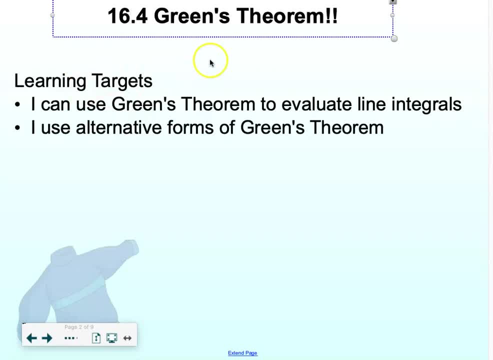 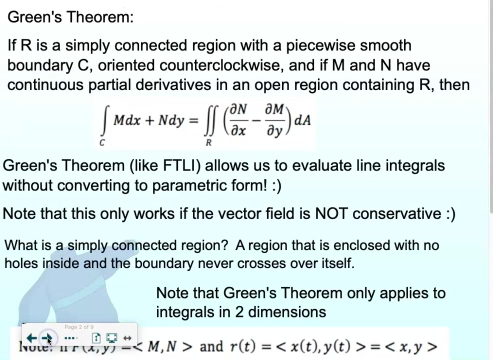 I just keep forgetting this little title thing. So anyway, there we go. Sixteen four Green theorem- Green theorem- All right, everyone ready? Sixteen four green theorem: Si: are you ready? All right, If R is a simply connected region with a piecewise, smooth boundary, C oriented counterclockwise, 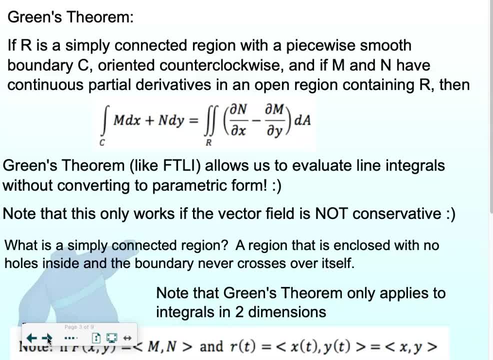 and if M and N have continuous partial derivatives in an open region containing R, then the line integral of MDX plus NDY is equal to the double integral of partial N, partial X minus partial M, partial Y over the area of the region. It's really action. 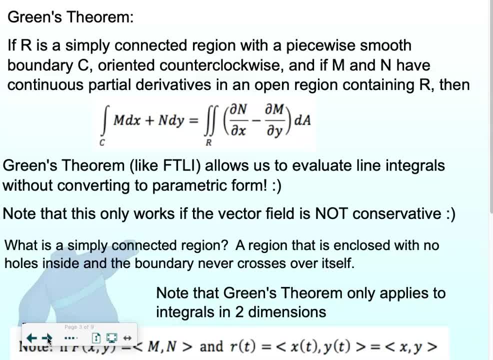 Okay, so here's the thing. So Green's theorem again allows us to evaluate line integrals without having to convert to parametric form. Note: Green's theorem only works if the vector field is not conservative, Because if the vector field is conservative, what would this equal? 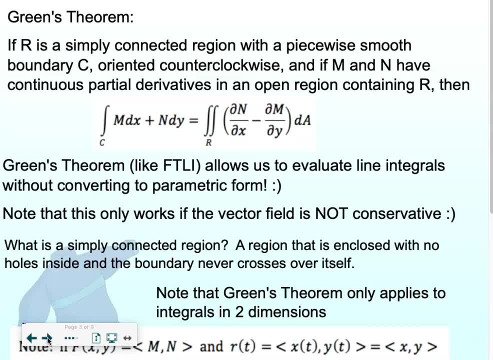 Zero, Zero, right, Okay, It's this right here. The integrand for Green's theorem is the exact same as your test for conservative. All right, Okay. a simply connected region is a region, basically, with a boundary that doesn't cross over itself and doesn't have any gaps. 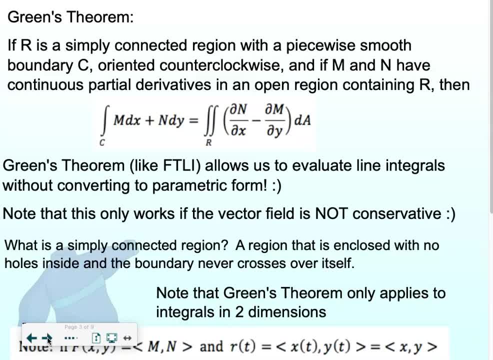 So it's a region where you can draw the boundary without lifting your petal And it never crosses over itself. So nice, simply connected region: No holes inside, no crossovers. So Green's theorem only works in two dimensions. Stokes' theorem is basically Green's theorem in three dimensions. 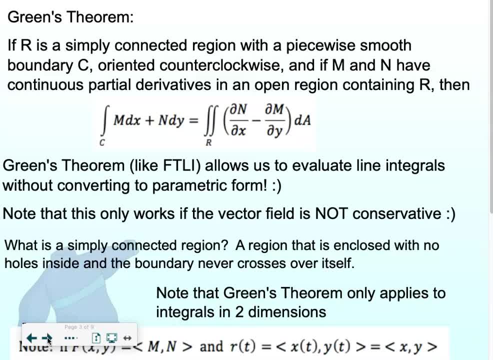 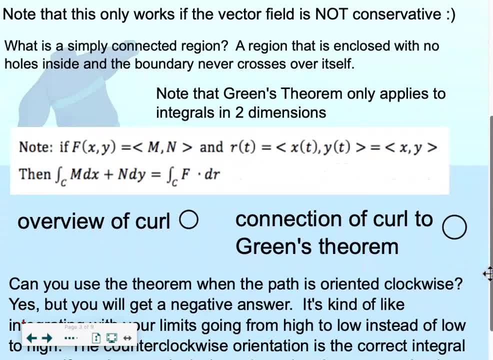 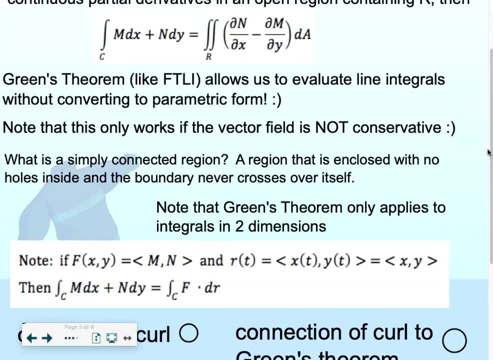 Don't forget: on the last set of slides we already pointed out that the line in a goal over some perc of MDX plus NDY is equivalent to F dot, DR. So now we know that that is also equivalent to partial, and partialized minus partial. 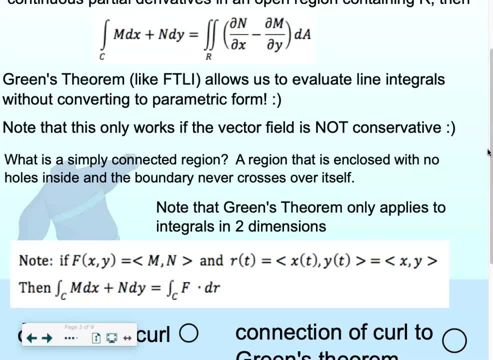 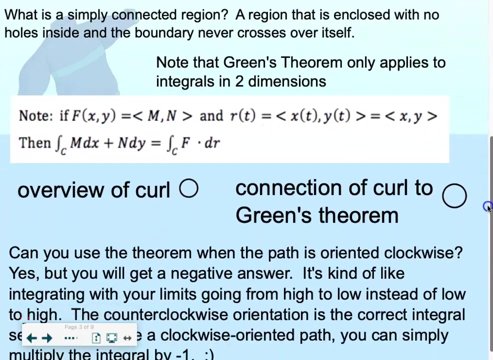 and partialized VA. So we're actually going to get back to the habit for today of writing double integrals that produce an area of a region. Okay, Okay, All right, Tell me if it's okay for me to scroll. You're done, Okay. 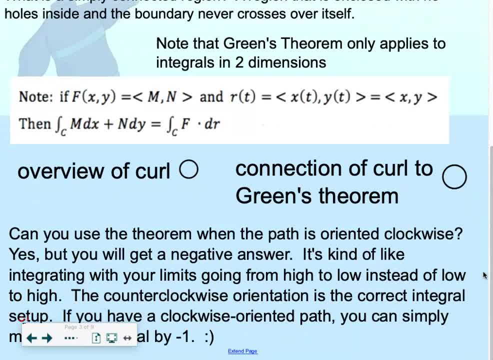 All right, Can you use the theorem when the path is oriented clockwise? Why does the path have to be oriented counterclockwise? Oriented counterclockwise, the way that they talk about- this a lot, A lot of mathematicians talk about. 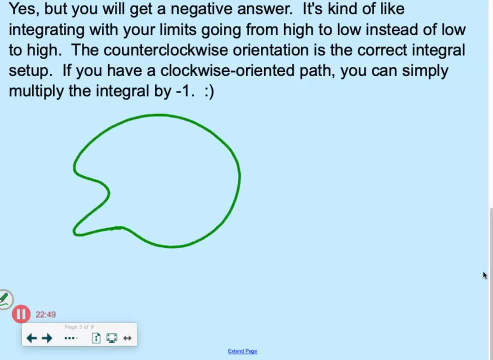 this. I don't know if your book says it like this or not, but it like say this is our curve key right Has to be simply connected, Has to be a closed region like it's all enclosed right. So if we have some simply 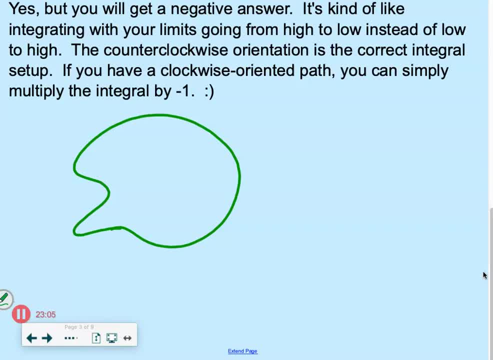 connected path. that means that if we were to walk along the path, the region that's enclosed would always be on our left. So when they say it's a counterclockwise oriented region, that's what they mean Is if you're walking along the boundary. 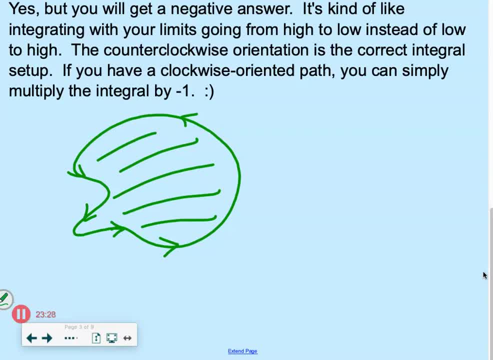 the region. the stop is always on your left. Now I have a student who actually asked the question. can't we do it? I mean, would the math be that different if it was clockwise oriented instead of counterclockwise oriented? 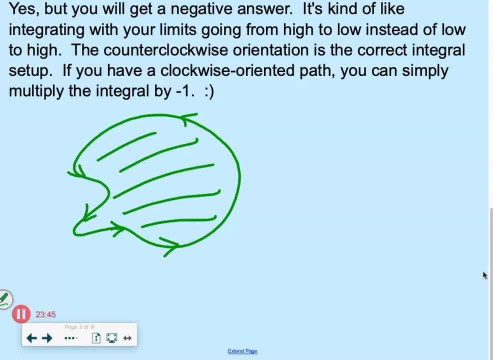 No, you'd actually get the exact same answer, Just negative. So if you have a clockwise oriented path, you're going to end up. you get the exact same answer, just times negative one. And that's OK. Just know that if you want to answer the question. 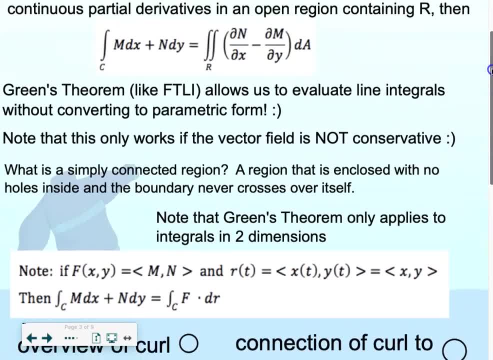 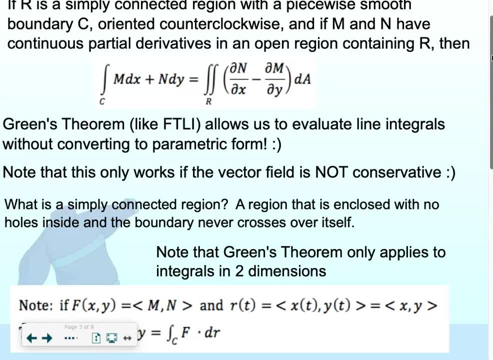 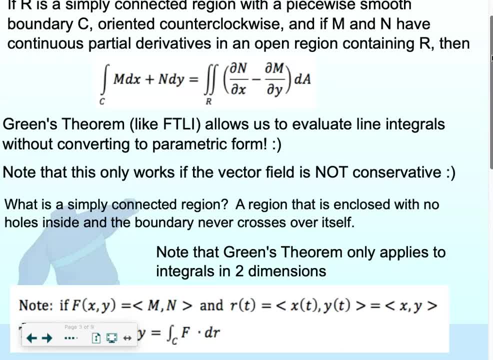 if your path is oriented counterclockwise, you get this theorem will give you the work. If it's oriented clockwise, then you got them all times by negative. How, what They have to give you a picture of what's up or tell me: all right. 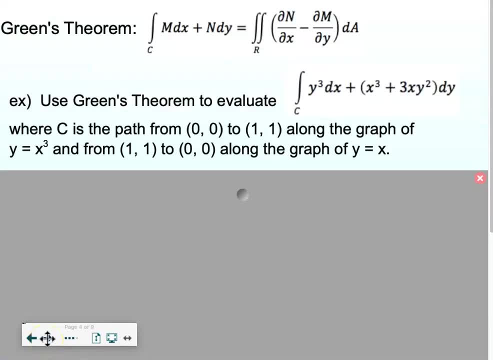 OK, So I'm retyping cinq terrains right there. So we're going to use Green's Theorem to evaluate the integral over the curve C of y cubed, vx plus x cubed plus 3y squared vy. C is the path from 0, 0 to 1, 1 along y equals x cubed and 1, 1 to 0, 0 along the graph of y equals x. 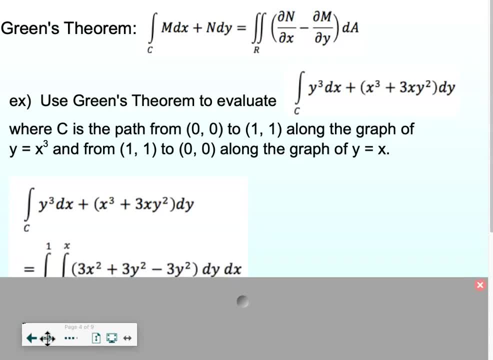 Personally, I would start by sketching my root. All right, so we're going to move this over and draw a sketch, All right. so 0, 0 to 1, 1 along y equals x cubed, and then 1, 1 to 0, 0 along y equals x not drawn to scale. 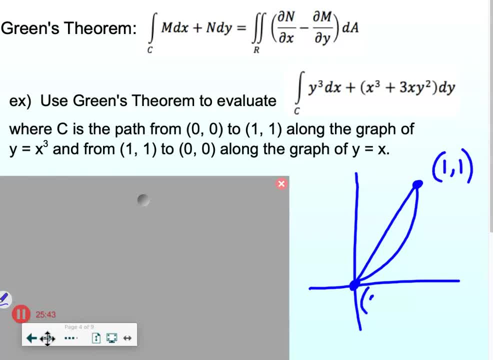 So here's 1, 1,. here's 0, 0, this is y equals x. cubed, this is y equals x- Rather than having to figure out this path in parametric form, which really wouldn't be that hard. 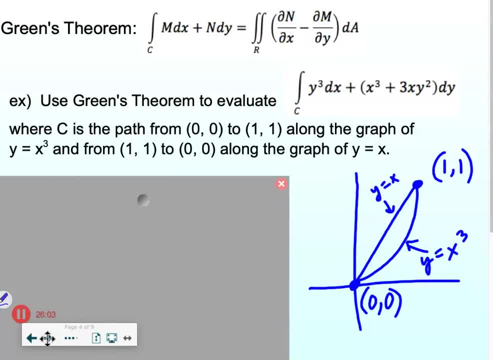 but rather than having to figure it out and remember, we're going this way: 0, 0 to 1, 1 along the x cubed, and then this way: 1, 1.. 1 to 0, 0 along y equals x. we are counterclockwise oriented on a simple connected region, right. 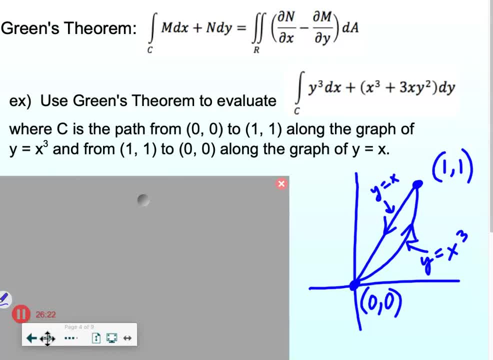 Okay. so rather than sitting there and converting these to parametric and converting that also to parametric and then doing an f? dot vr, instead we can apply Green's Theorem over the double integral that gives us the area of this region. Okay. 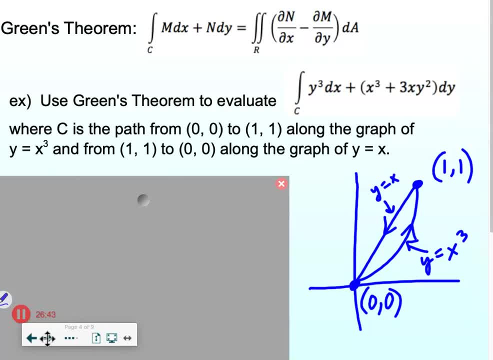 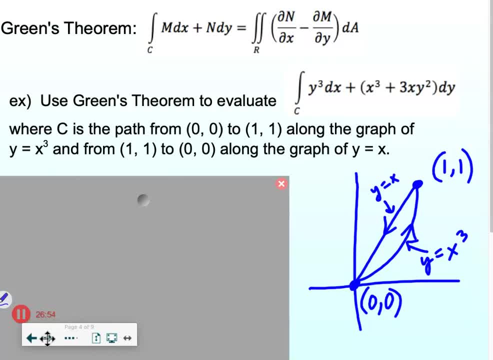 Top right side, Right, All right, So, oh, but we got to do- oh, that's just me sitting here, All right, So to set up the integrand so you have to do dn, dx, plus or minus dn. let me see what's right. 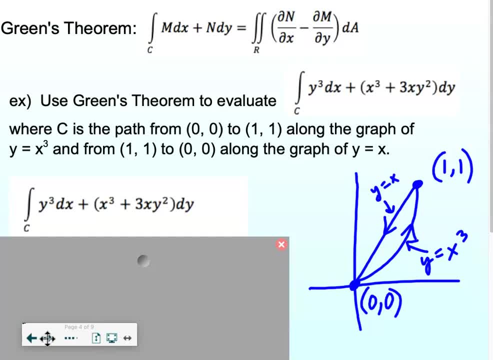 The n dx minus the m dy. So if you want to go ahead and take a minute and find, like the guts of your integrand your Green's part, So partial n, partial x minus partial m, partial y, This would be. this is like your m and this is your m. 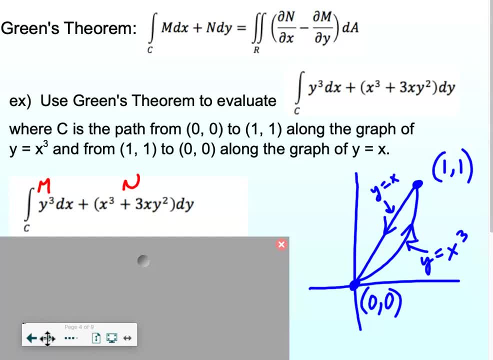 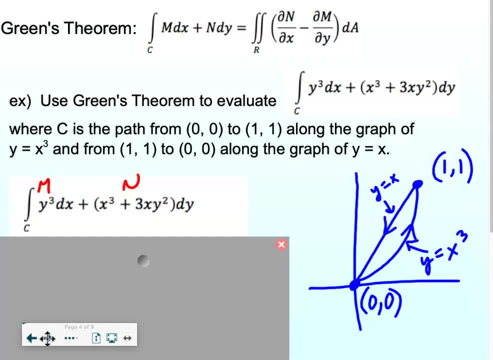 so the green part. then partial n, partial x would be 3x squared plus 3y squared, and then partial m, partial y would be 3y squared. so you have 3x squared plus 3y squared, minus 3y squared, and then dy, dx, and then your limits of your integrand are the limits that give you the area. 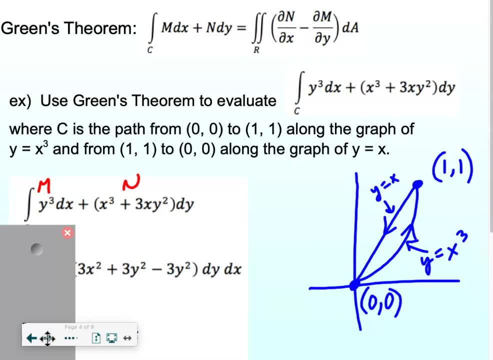 of that region, which now, whenever we have a region of this shape in ap prop, i'm calling it so- the area of our integral. so you should have um, x going from 0 to 1 and y going from x to x. then clean up your integral, go ahead and evaluate. 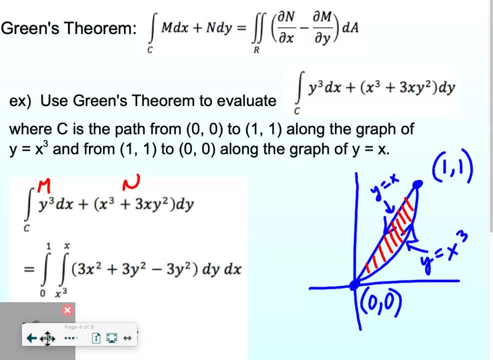 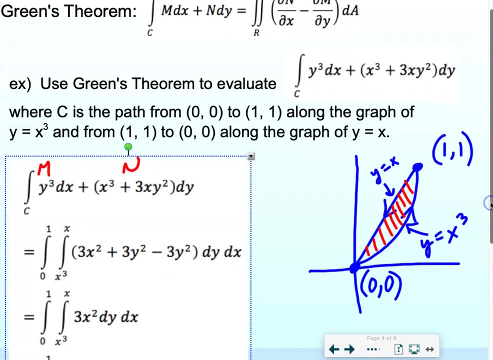 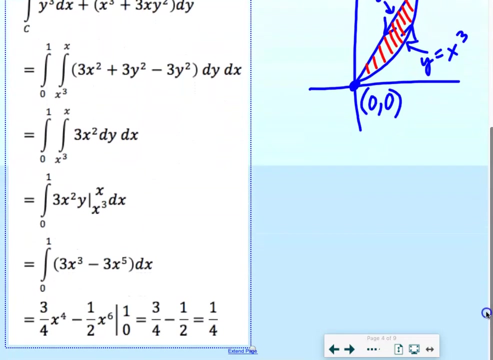 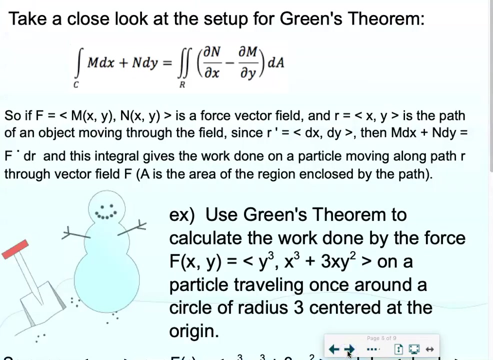 you do like a breath of fresh air. I don't know if that's the end, Thank you. Thank you, All right, good. So this is me just reiterating again that this is easy. This is easy. Equal to f dot dr. 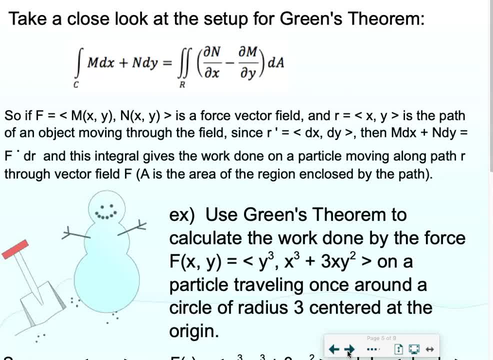 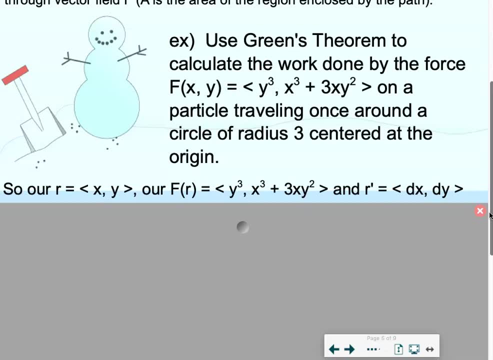 So again, this gives even Green's theorem gives the work done on a particle moving along path r through vector field f. That's just me saying that again, Okay, All right, Use Green's theorem to calculate the work done by the force f, big F of x, y. 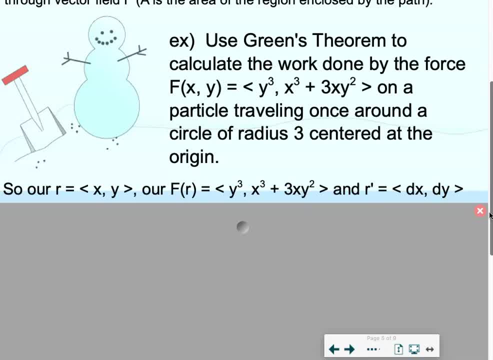 equals y cubed, x cubed plus 3xy, squared on a particle traveling once around a circle- I almost said surface, around a circle of radius three, centered at the origin. Centered at the origin, So your path, notice. it didn't say traveling counterclockwise. 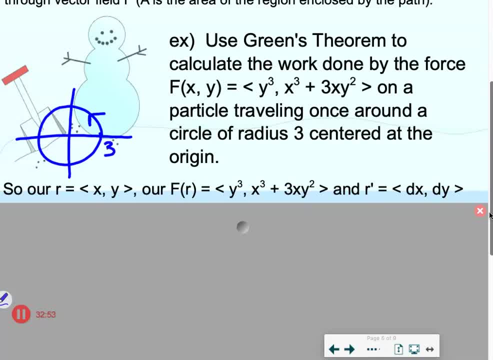 Let's make it counterclockwise: Circle of radius three, centered at the origin. So there's your path. Remember Green's theorem. You just need the air like it's the double integral Over the area. If you want to keep this with x's and y's, that's fine. 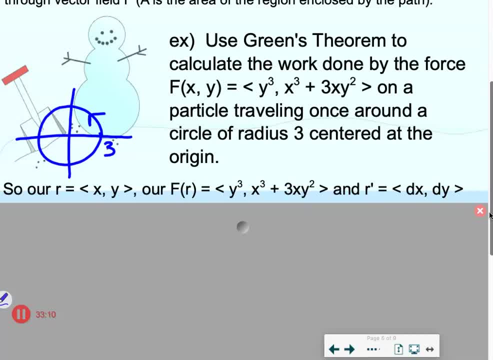 If you want to convert it to polar, that's fine. So whatever you prefer, But you might want to do your d- how do I say this? d, d, dn, dx minus, dm, dy first And then do a polar conversion if you want to convert to polar. 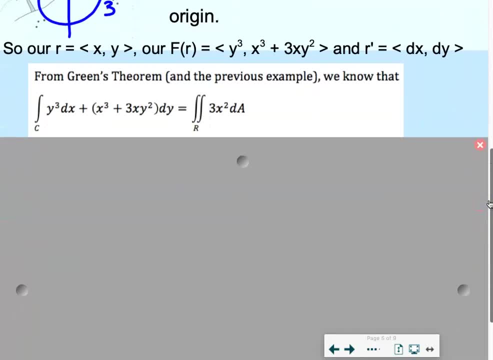 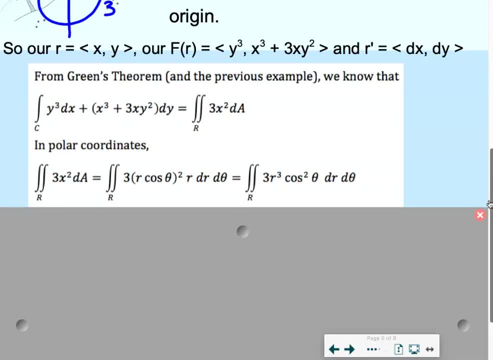 So we have 3x squared evaluated over the integral. So this is the, the integral, as r just goes from zero to. why did I not do the limits right away? r goes from zero to three. theta goes from zero to two pi. 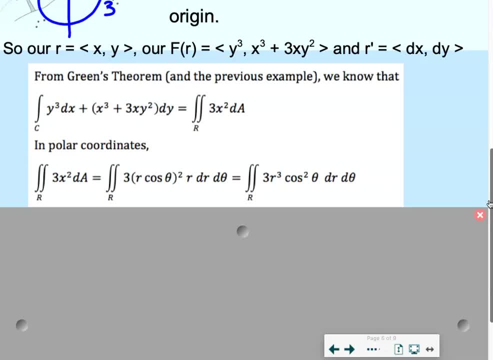 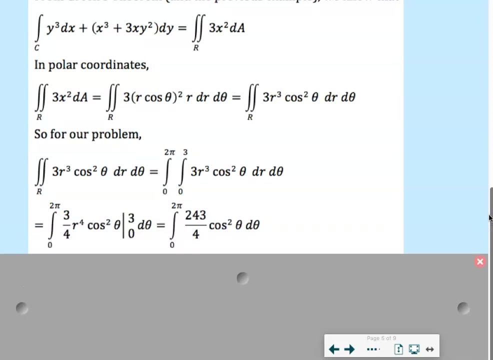 And remember it's x is r cosine theta times r dr d theta right. So I just cleaned that up and then apparently waited four steps to put my limits on. So there we go, All right. So, and I differentiate dr. 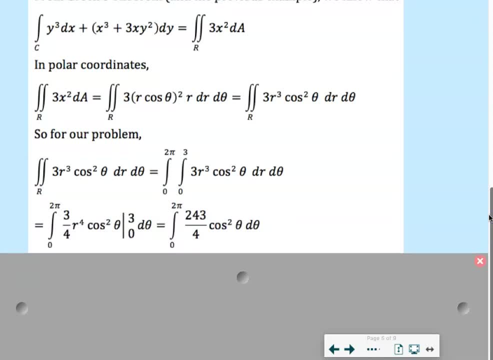 So three-fourths over the fourth, plug in, plug in, you get this guy Anti-derivative of cosine squared. you have to do a power reduction So you end up with one-half times one plus cosine, two theta. And we anti-differentiate cosine two theta. anti-derivative is two sine or one-half sine two theta. 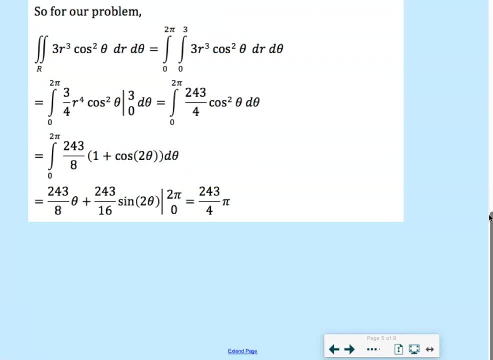 So you end up with two-hundred-forty-thirds fourths pi. Is that what you got? Okay, Did you? Yay, You messed up twice, but you got it. Oh yeah, Okay, All right. The main part that I want to make sure you learn is the setup right. 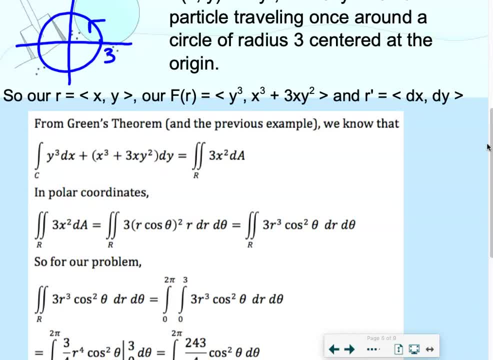 So do you understand how to convert from the f, the big vector field, to apply Green's theorem And then setting up area is what we did last chapter, So I'm not worried about that. Most of you can do an area just fine. 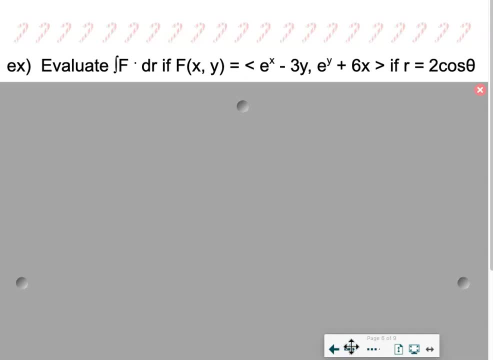 Here's another one just for fun. So evaluate f dot t, F dot t r. if your vector field is e to the x- because I thought I'd be good at this- e to the x minus 3y comma. e to the y plus 6x. 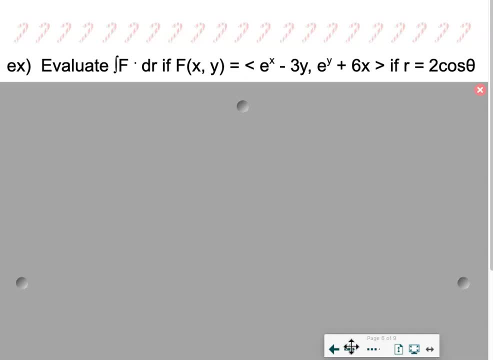 If your r, your path is two cosine theta, why do I not have any limits? Maybe you should just go back. You think there's more? No, No, No, Nope. What's the Green's theorem? I think I just have it. looks like I just intended for you guys to do it from high house. 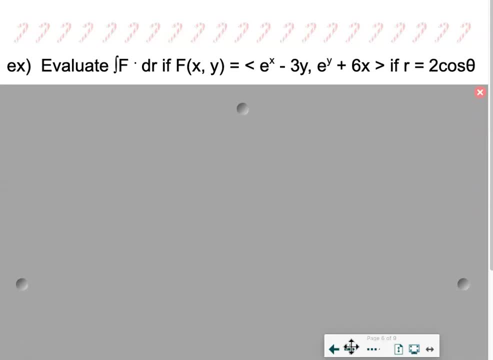 to free high house, but I'm not sure. Oh, this is a polar equation. This isn't: y equals cosine two cosine x. This is r equals two cosine theta. This is already in polar form. It's already defined for you in polar form. 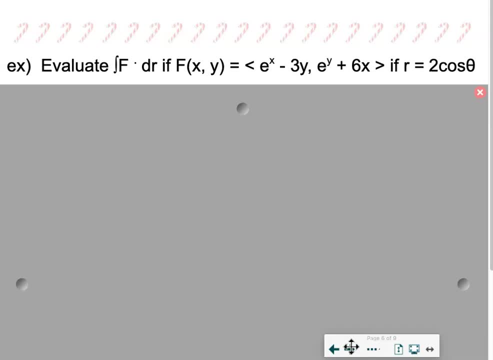 So we have a lovely polar equation: R equals two cosine theta. So see if you can write your Green's theorem. set up and see if you can grasp this in polar form. Find your limit Right. You can do this. At least do the set up. 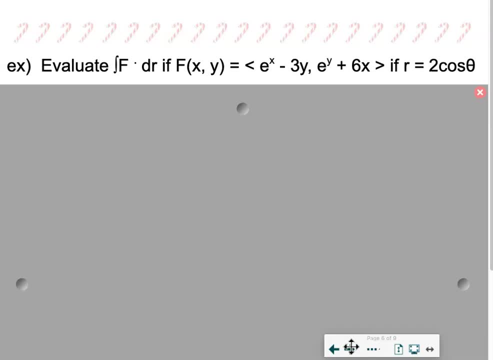 You don't have to evaluate, Do the set up. So do you guys remember two cosine theta: It's when, and now plot points, right? That's what my geometry teacher always used to say. So you want to find out what your R is.